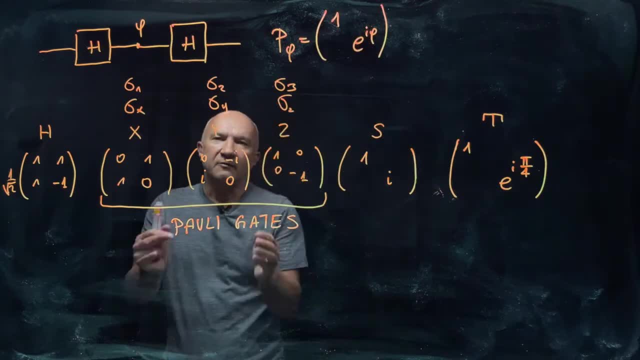 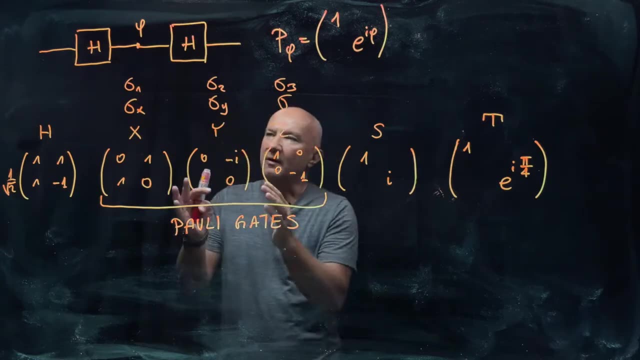 So it's a special form of the phase gate. Now, the Y gate is a product of, essentially a product of- X and Z. They will play a substantial role in just everything. we'll be talking about everything related to a single qubit. So one reason being, for example, that X, Y and Z, plus the identity, 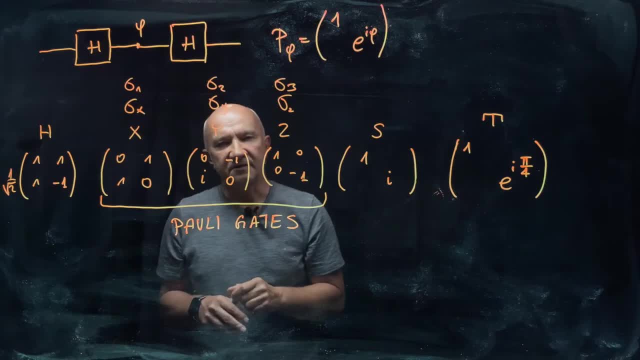 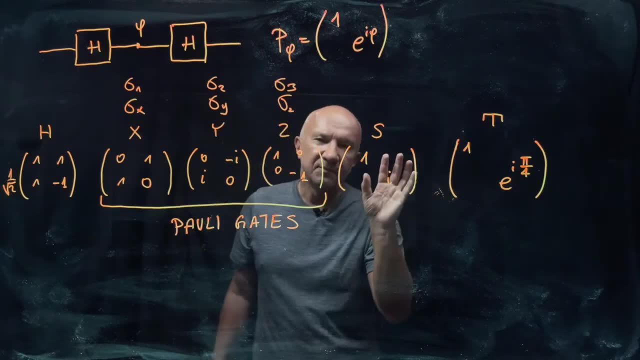 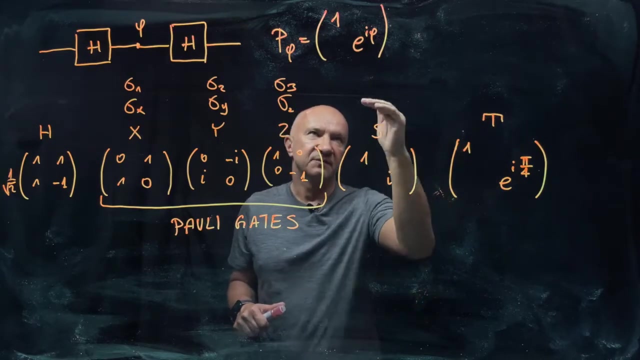 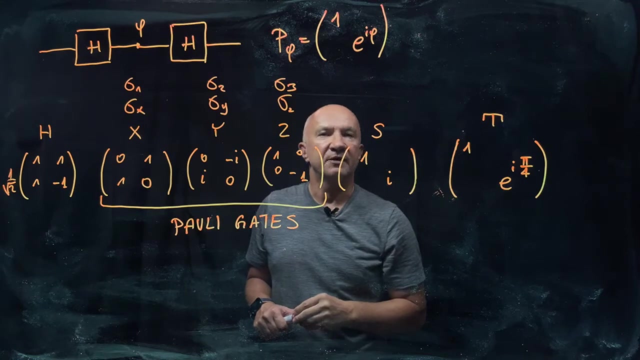 matrix form a very useful and very convenient basis in the set of all 2 by 2 matrices. Another two phase gates that require special mention is the S gate and the T gate. So the S gate is Again a special case of the phase gate, with the phase shift equal to pi over 2.. And the 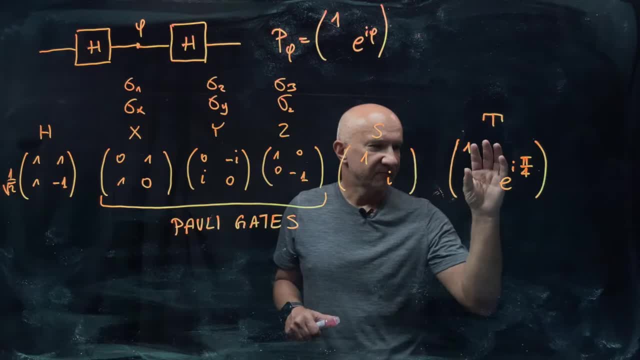 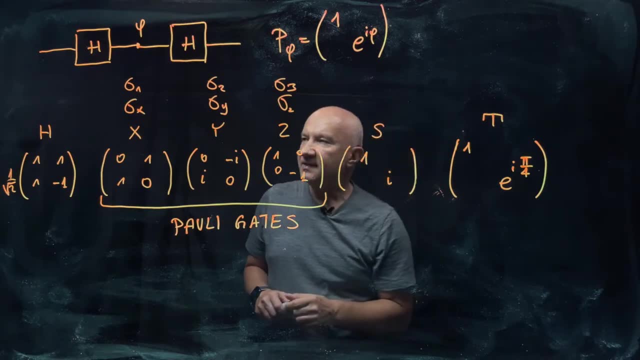 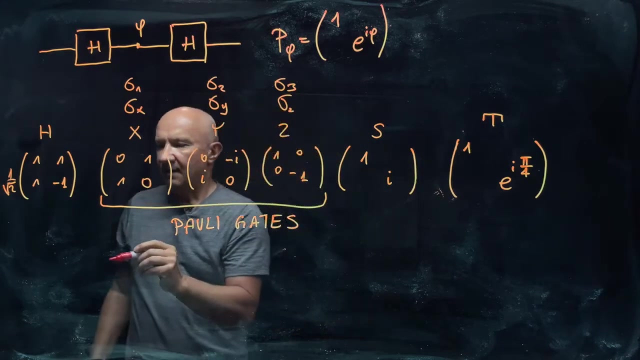 T gate is the special case of the phase gate, with a phase shift phi equal to pi over 4.. Now, as it happens, the Hadamard, the Pauli matrices, the Pauli gates and the S gate form another interesting set. 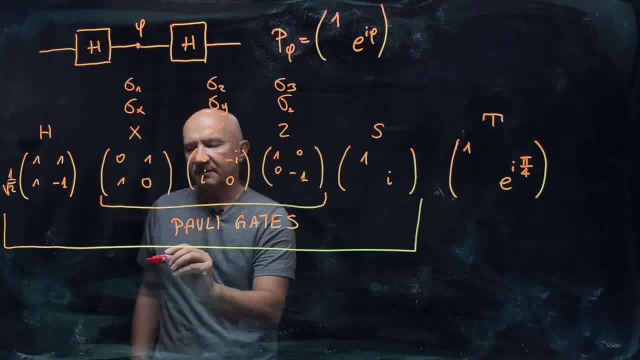 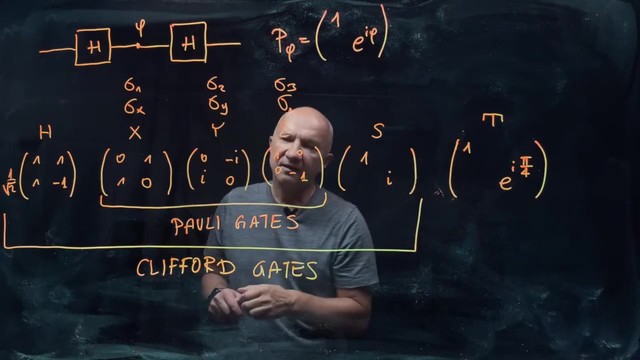 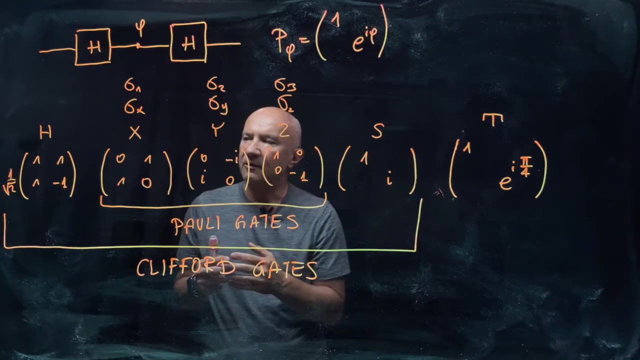 But we call this a set of single qubit gates, the Clifford gates on the single qubit. So Clifford gates Again. we will talk about them later on when we'll talk about quantum error correction, but also when we talk about how easy it is to simulate quantum computation on classical 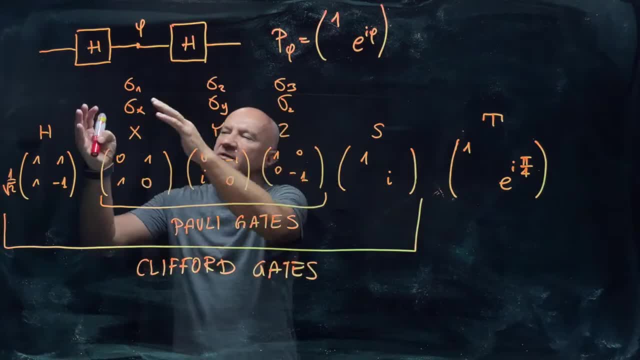 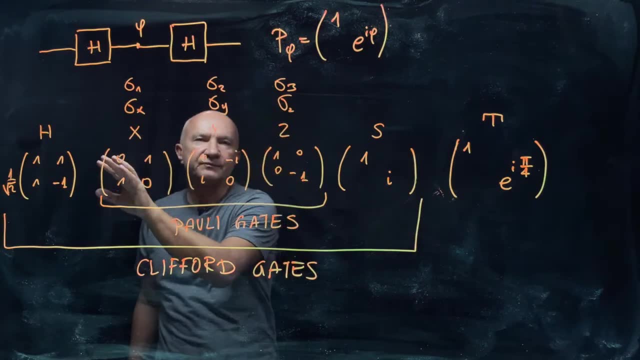 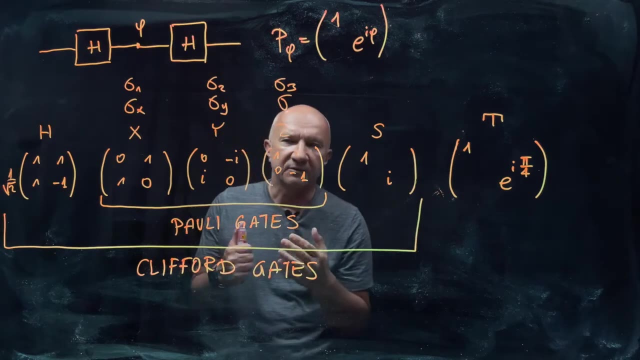 devices. So, as it happens, if all the set of possible operations on a single qubit were to be restricted to this set of 5 gates, then it would actually be quite easy to simulate quantum computation on a classical device. So somehow the set of operation that they generate is not too rich, But nonetheless. 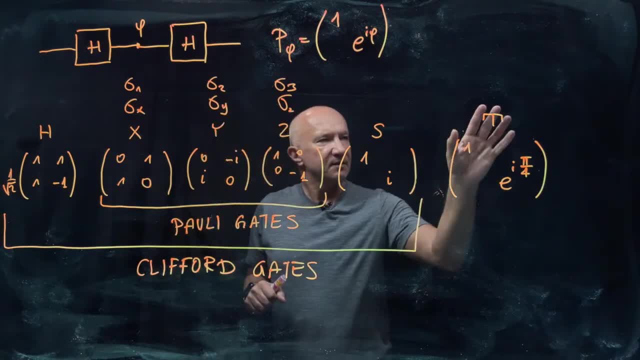 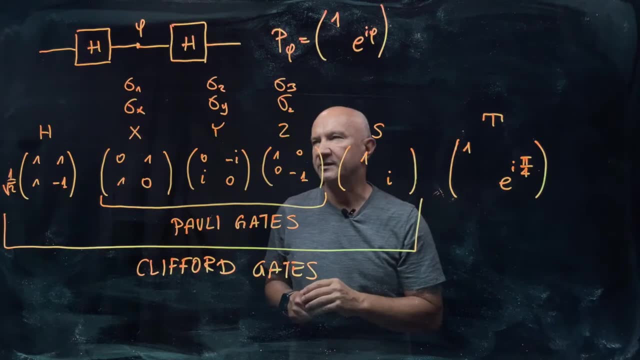 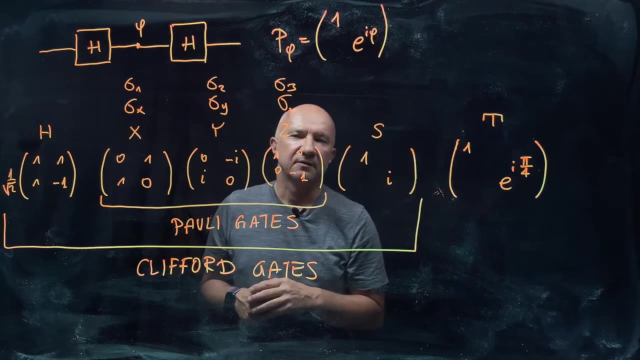 it's a very important set of gates. So the T gate is outside this Clifford set for a single qubit operation and it's actually quite important because it will just allow us to explore the whole richness of operations on the set of all unitary operations on a single qubit.